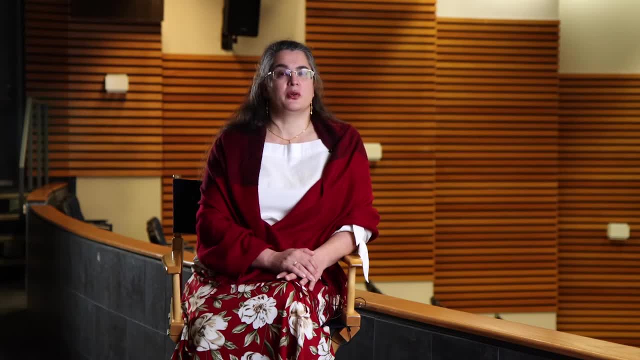 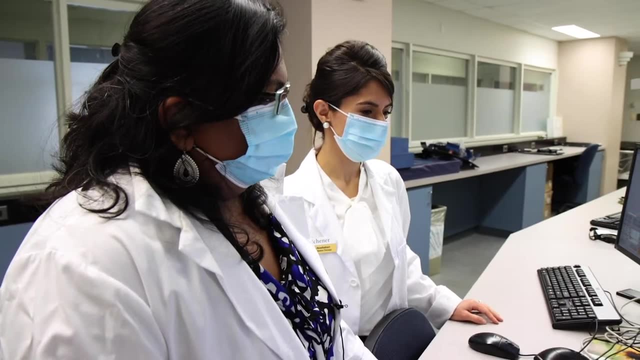 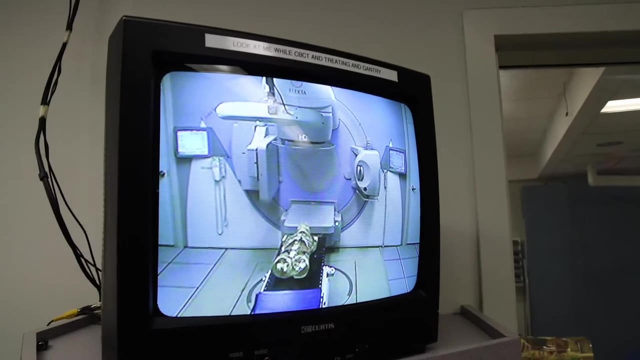 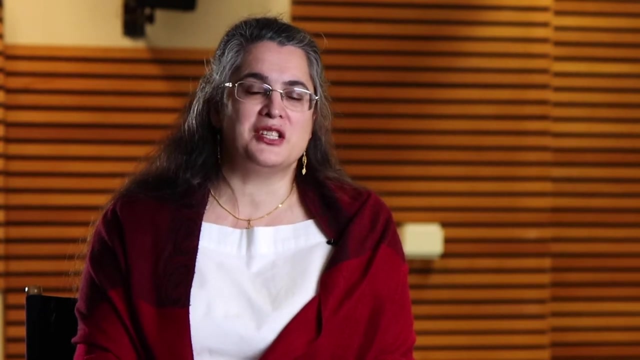 within my portfolio two Radiation Therapy programs, One joint with the University of Toronto as part of the Medical Radiation Sciences joint program and one focused more on the needs of Northern Ontario, so that is joint with our Laurentian University partner. I really want to thank you and encourage you to attend the sessions in Radiation Therapy and MRI and 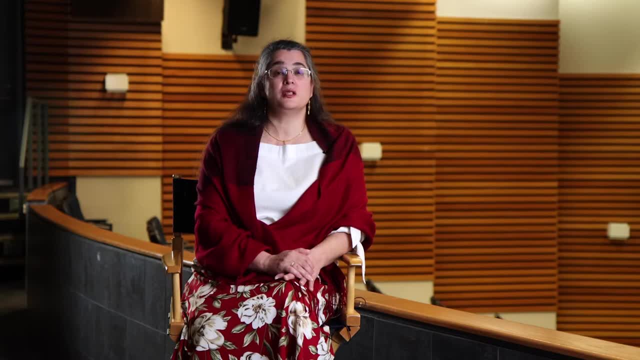 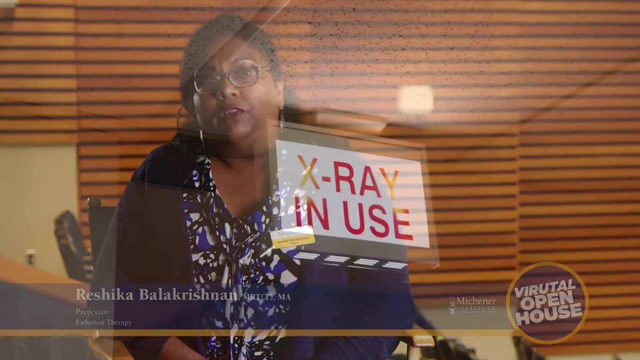 looking forward to seeing you as potentially future colleagues. Take care, I'm Rishika Balakrishnan, faculty at the Michener Institute in the Radiation Therapy program. You're considering a program in health care at the right time. Every contribution that 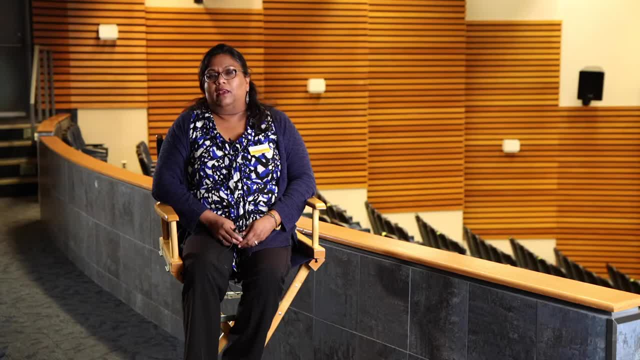 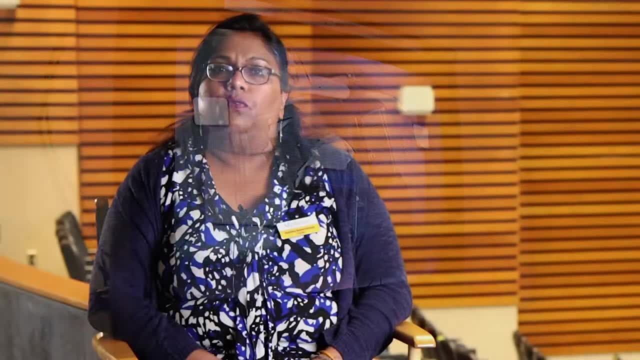 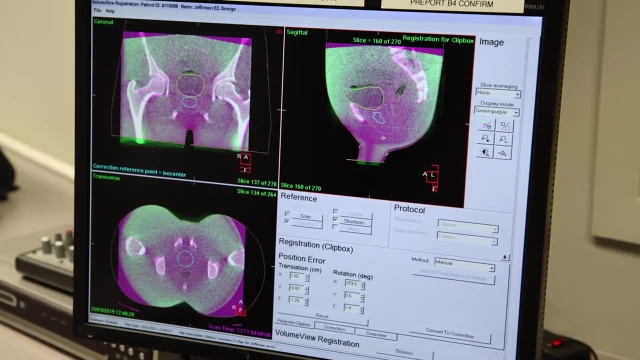 you make in health care makes a phenomenal impact in today's society. The Michener Institute provides programs for both Laurentian University as well as for University of Toronto. The program admission requirements are different for both of these programs. The interesting aspect of this program is that it is direct entry from high school. The requirements: 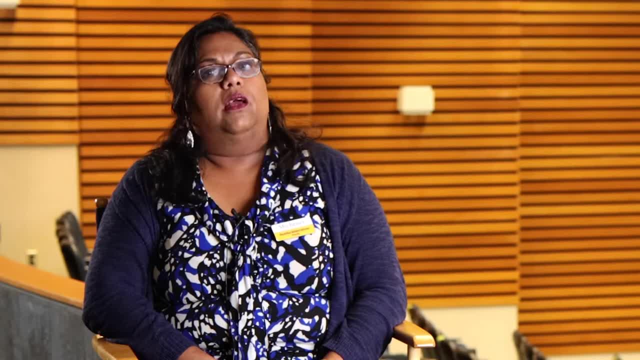 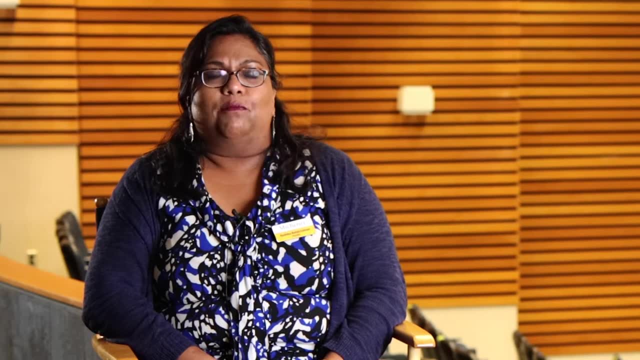 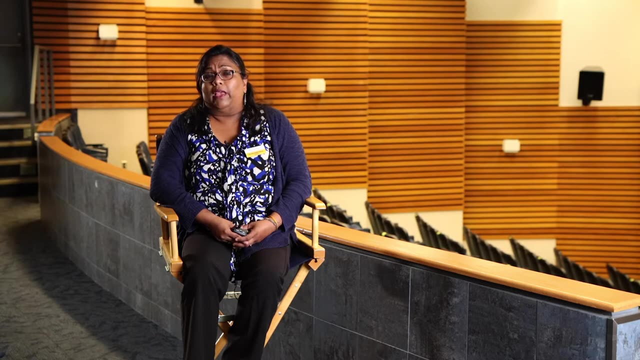 to enter into this program is a high school diploma, along with a minimum of six university level courses. The program on its own has many forms of instruction that is being given. One of the interesting aspects is that you will have in-person classes at the Laurentian University. 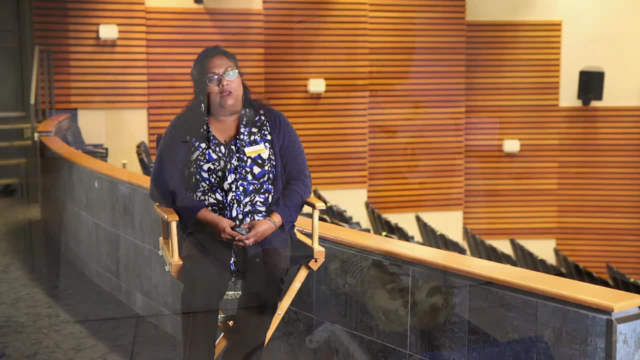 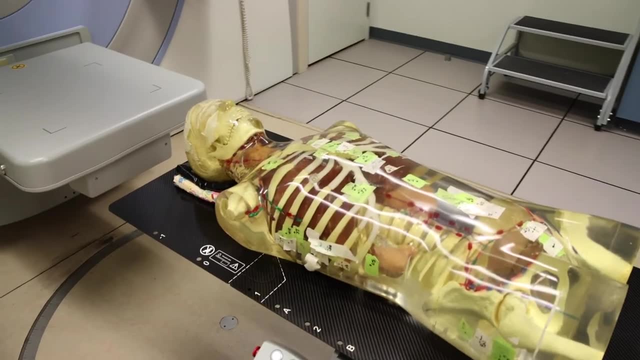 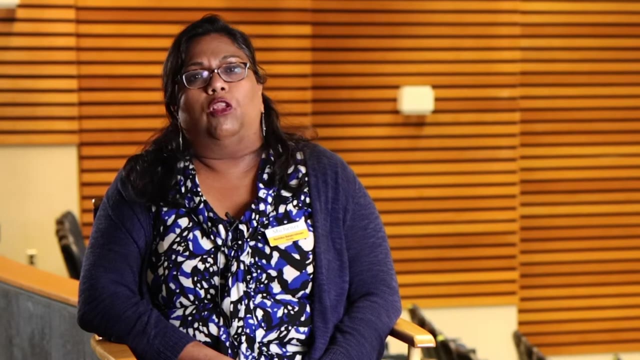 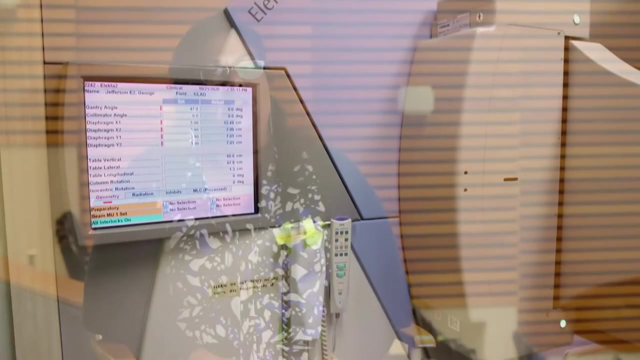 in Sudbury. The program has a clinical component where our students will be placed in a clinical hospital affiliated with the program where they'll get to work with radiation therapists alongside the rest of the team. Radiation therapists work very closely with a team of professionals. We tend to 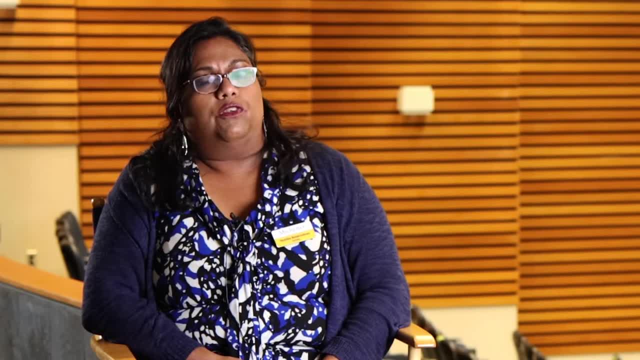 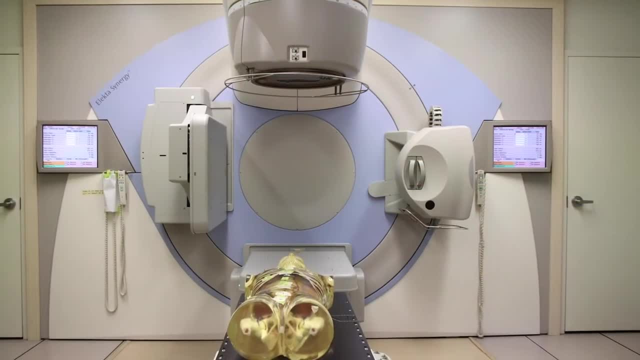 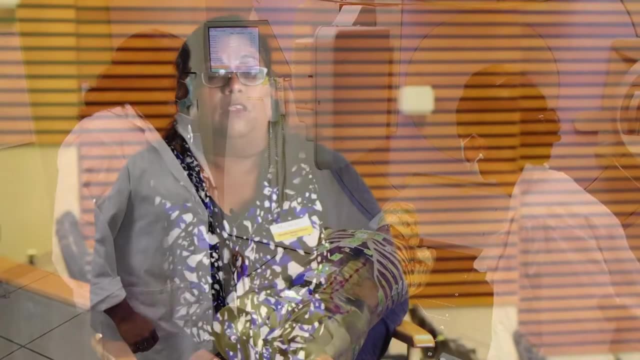 work with radiation oncologists, physicists, nurses and other fellow allied health professionals. We use advanced computer systems and sophisticated radiation therapy equipment to deliver radiation to our patients. It involves a lot of technical work as well as patient care, where you are talking to people. 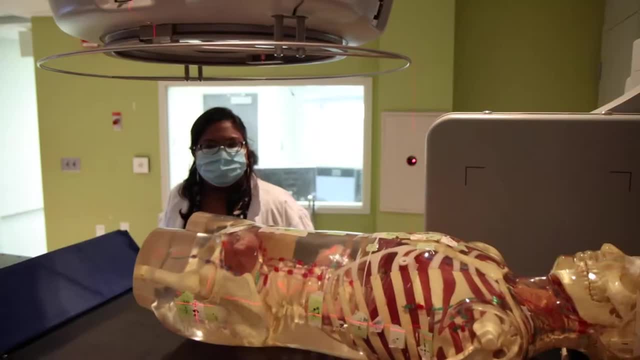 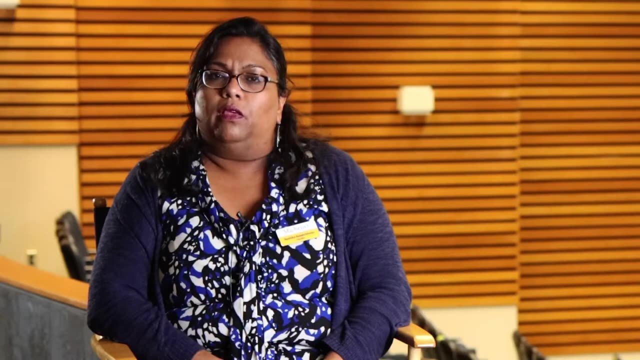 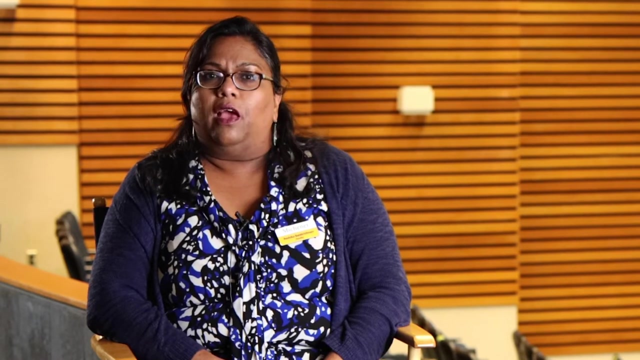 and helping them through a very difficult time in their lives. The work is fast paced, diverse and involves a lot of interpersonal communication skills with not only the patient, but also with their families. A good portion of our time is spent talking to the patients, as well as their families. 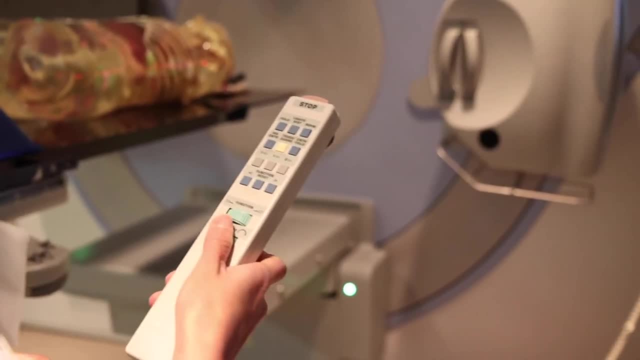 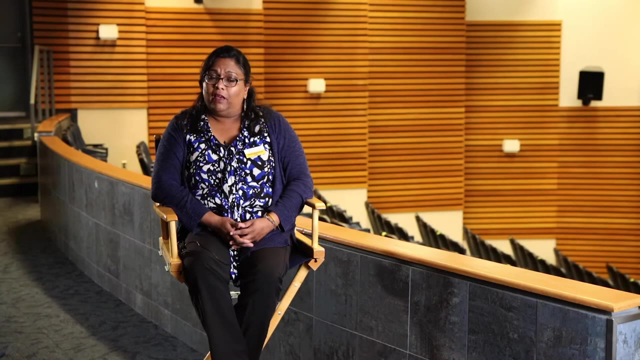 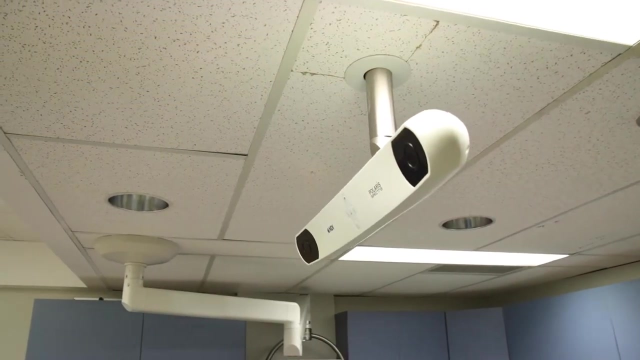 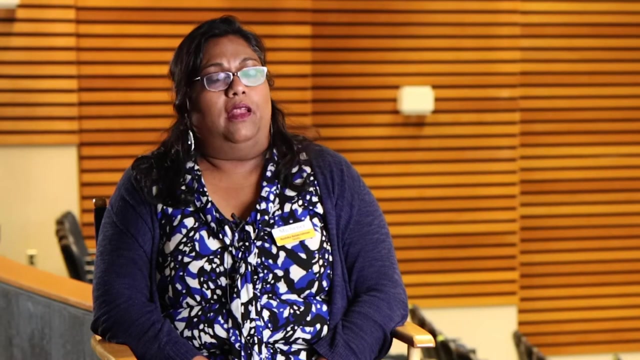 helping them address their concerns as they go along treatments. If you like, the idea of playing a vital role in healthcare, working alongside with patients and other healthcare professionals. excellent communication skills. you're looking at a very appropriate program for yourselves. You want to play a vital role in a patient's cancer treatment, a strong communicator and 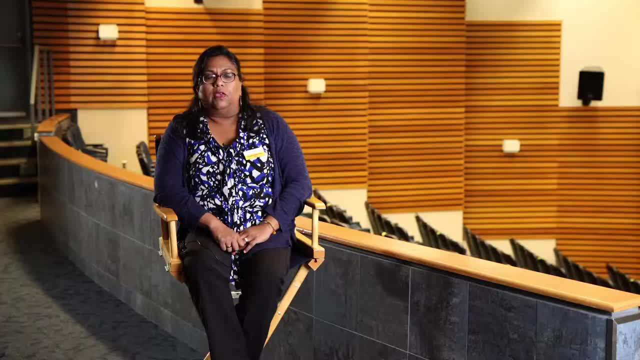 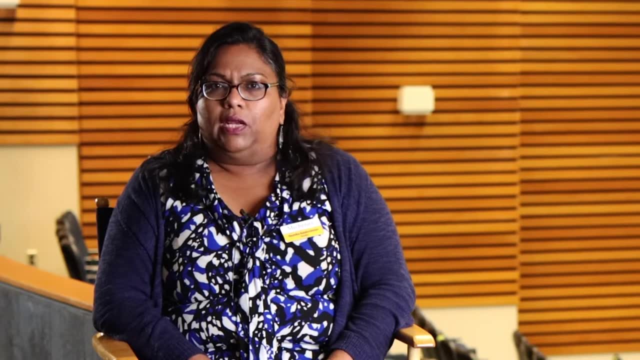 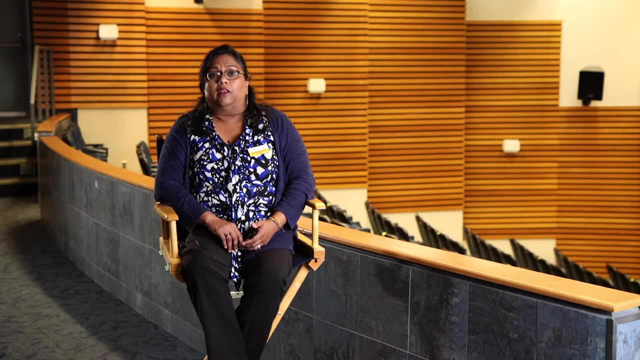 have an apt for computers and technological programs, radiation therapy might be a good fit for you. Whether it's designing a treatment plan, applying radiation or supporting our patients through their treatments, you're providing a vital role in their lives and contributing to their lives tremendously. 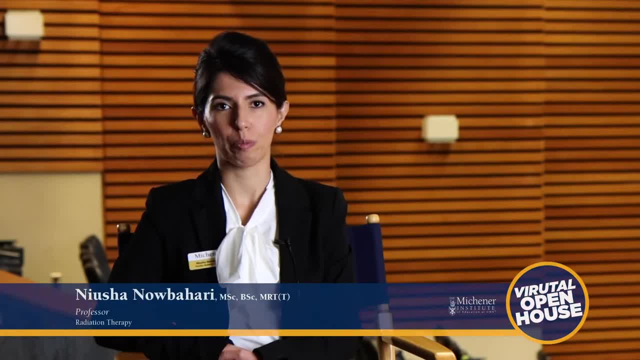 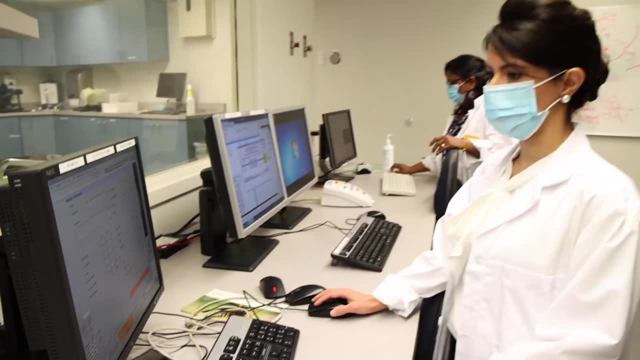 My name is Neushan Obahari. I'm a faculty member in the radiation therapy program at Michener In our joint program with the University of Toronto. Until you earn an advanced diploma from the Michener, you'll also earn a Bachelor of. 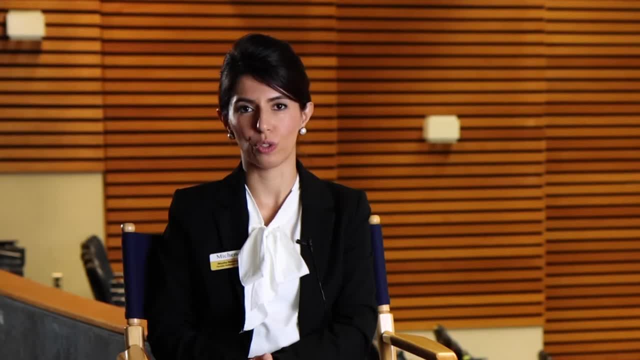 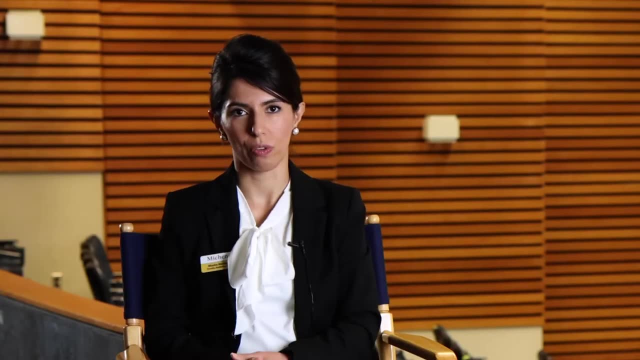 Science degree in Medical Radiation Sciences from the University of Toronto's Faculty of Medicine. The University of Toronto joint program is what's referred to as a second entry program, which means you need at least one year of university education in order to apply into the program. 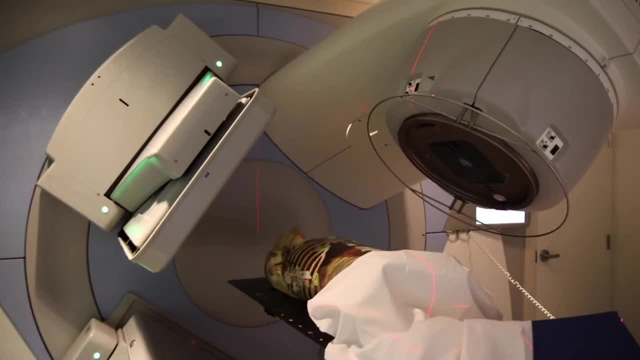 The program is a total of eight semesters done consecutively over a three year period, with onsite classes at both the Michener Institute and the University of Toronto. The program is a total of eight semesters done consecutively over a three year period, with onsite classes at both the Michener Institute and the University of Toronto. 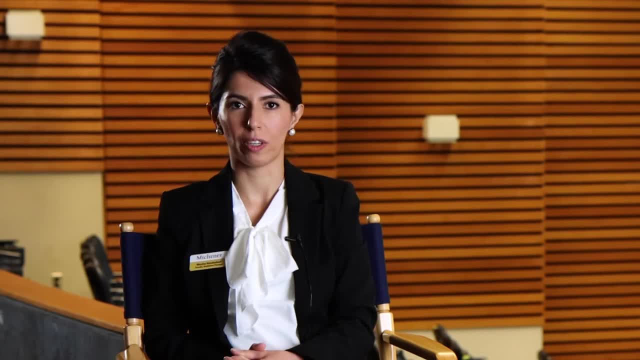 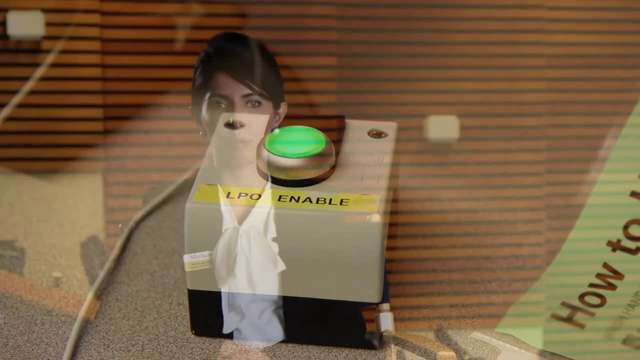 The program is a total of eight semesters done consecutively over a three year period, with onsite classes at both the Michener Institute and the University of Toronto And hands-on clinical experience at one of our affiliated cancer centres. Students learn through a a mixture of classroom time, hands-on laboratory activities and 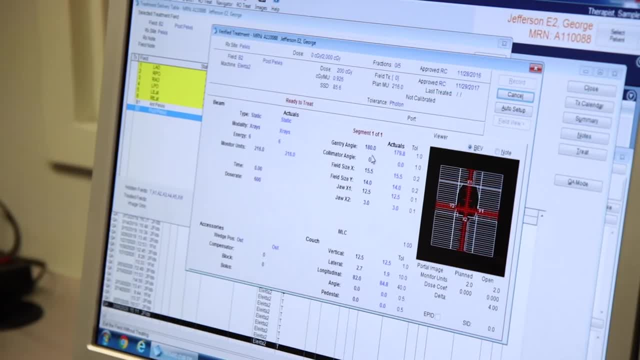 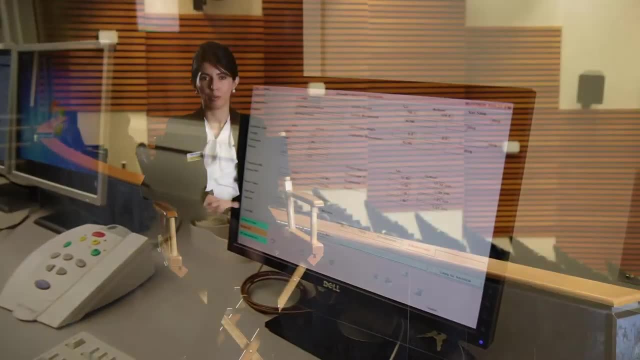 clinical experience with one of Michener's many affiliated health care partners. These placements prepare students to be job ready. students get the opportunity to network with potential future employers. For full details on admission requirements to both the Michener Laurence Hospital and St William's,